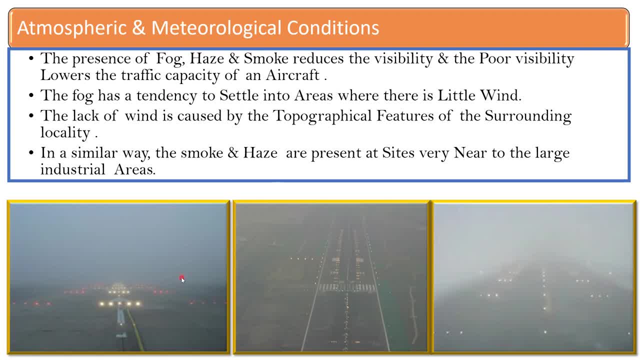 We have the construction, then we have ground accessibility, presence of other airports. we know this, Usually in the time of rainy season, or especially in the month of, you know, November, December, during the winter season, and all we usually encounter there is a delay of 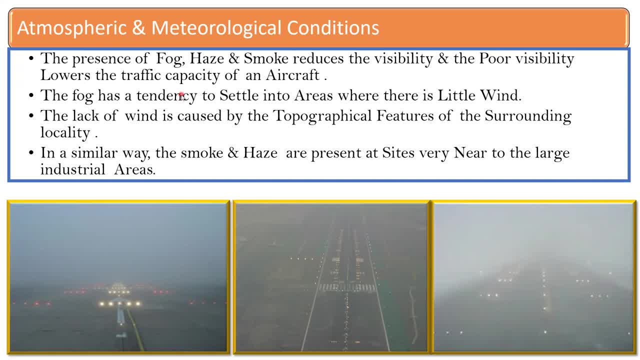 flight and all right. The main reason behind that is due to the fog and all. The second is the fog has a tendency to settle into the areas where there is a little wind. So, as a result of that, what will happen Sometimes? if you look at here, sometimes it will become difficult for the pilot. 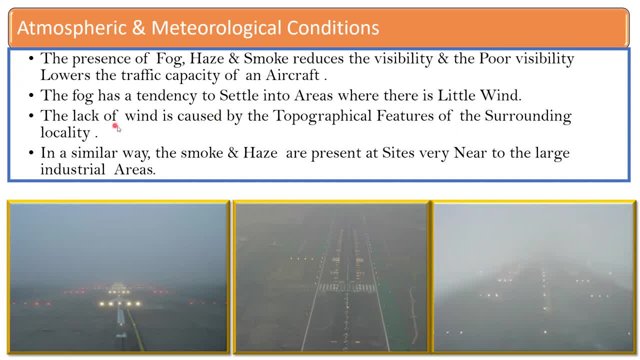 to do the landing operation. Next is the lack of wind is caused by the topographical features of the surrounding locality. In a similar way, the smoke and haze are presented sites very near to the large industrial areas right. So if you have a very 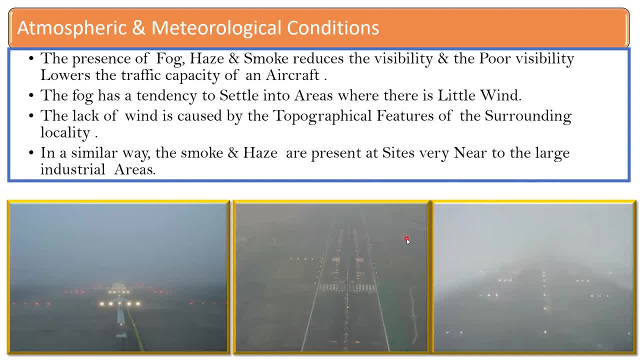 large industrial area in the nearby zone of airport, then, due to the smoke coming out from that industry, what will happen? There are chances of more fog being getting created. So that is why, whenever we try to put the airport, whenever we try to find the location for the airport, 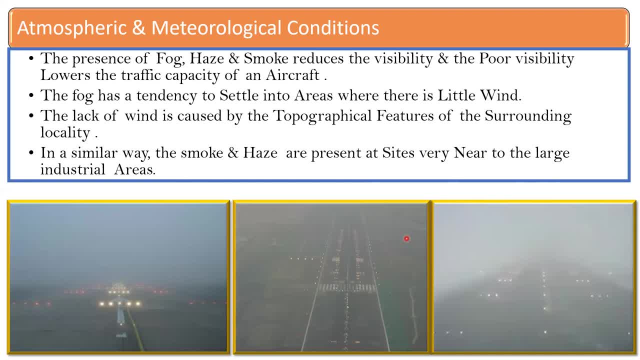 we should consider all these things in mind so that in the nearby we don't have any factories at all, So where the smoke will come out from that particular factory, and later it is going to create a problem for us, right? So this is the first thing that we need to consider. Next is availability of 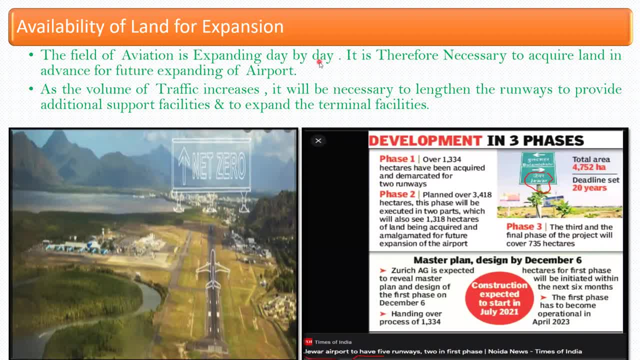 the land for expansion. The field of aviation is expanding day by day. It is therefore necessary to acquire land in advance for future expanding of the airport Has a volume of traffic increases, that is, a aircraft traffic increases. It will be necessary to lengthen the runways to provide 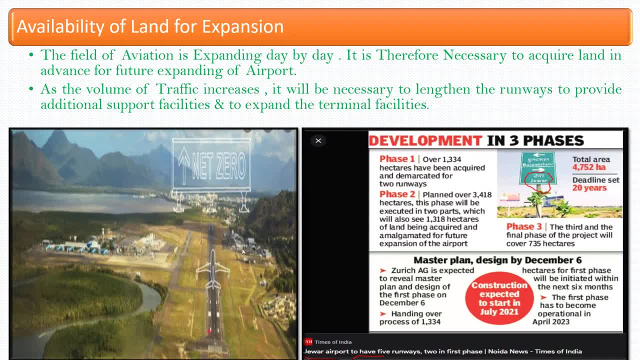 additional support facilities and to expand the terminal facilities. So whenever we try to acquire the land, we have to make sure that whatever land we have in the surrounding areas, those also will acquire that acquire so that in future we can go for the development. Now this is one of the articles. you can see it here: Jawer airport to have fire and. 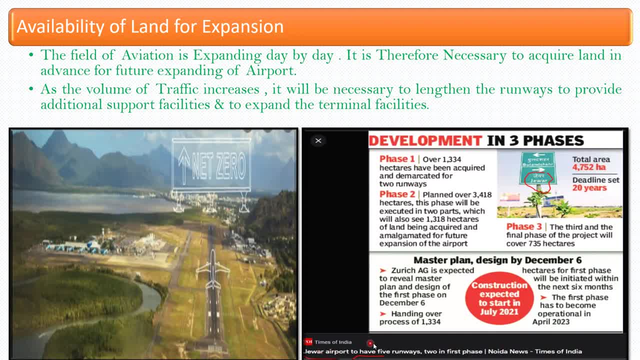 waste two in the first phase, right. So Jawer airport is coming up in Uttar Pradesh and this is how they are planning, actually right Development in three phases. So what they're going to do, they will acquire the land initially and then, phase-wise, they are going to acquire the land. 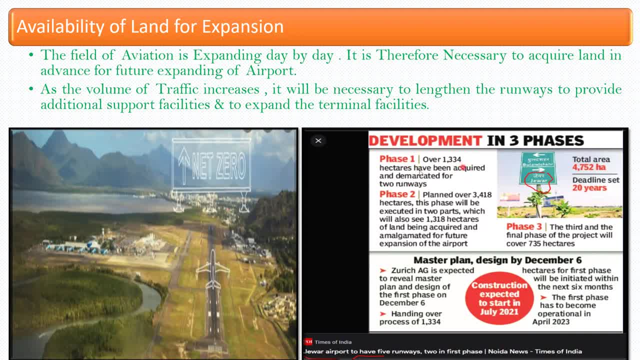 They are going to do the things. that is phase one. over 1,334 hectares have been acquired and demarcated for the two runways And all these things. usually what to try to find in the newspaper, And also you can see it here: the master plan, which is the design by December 6.. 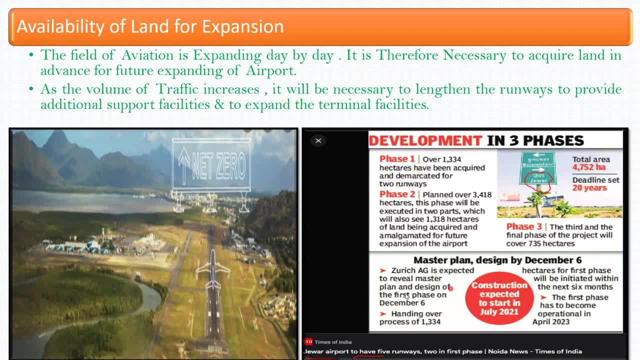 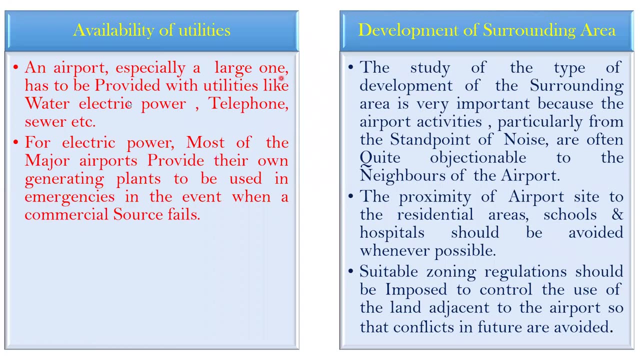 The Zurich AG is expected to reveal the master plan and design of the first phase on the December 6,, right? So they'll having a master plan and all And based on that the executions will be done. Yeah, So the next one is the availability of the utilities: An airport, especially a large one. 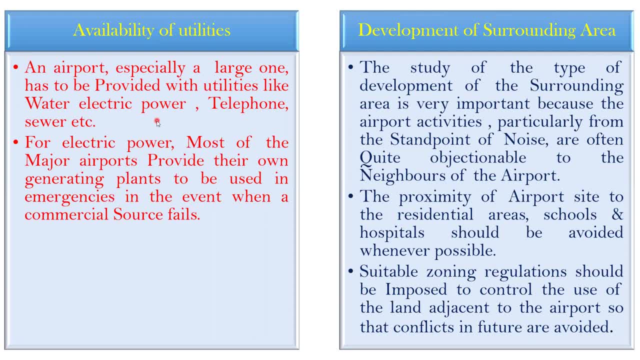 has to be provided with utilities like water, electric power, telephone, sewer lines, etc. For electric power, most of the major inputs provide their own generating plants to be used in the emergencies in the event when the commercial source fails. So again, this also plays a very important role for us, That is the telephone. 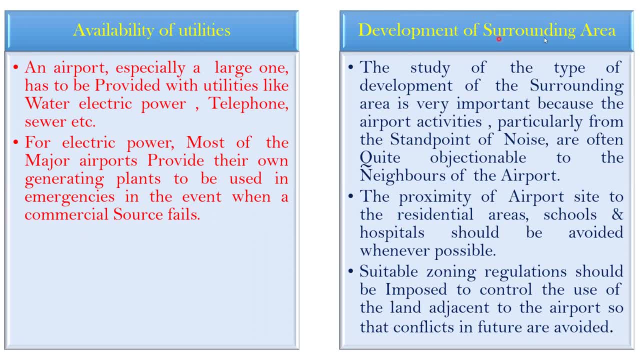 the sewer lines and all right. And next is the development of the surrounding area. The study of the type of development of the surrounding area is very important because the airport activities, particularly from the standpoint of noise, are often quite objectionable to the neighbours of 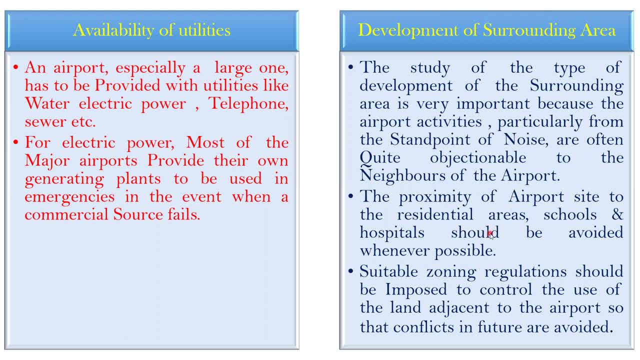 the airport. The proximity of the airport site to the residential area, schools and hospitals should be avoided whenever possible. We've already seen this also. Suitable zoning regulations should be imposed to control the use of land adjacent to the airport, So that the conflicts in future are. 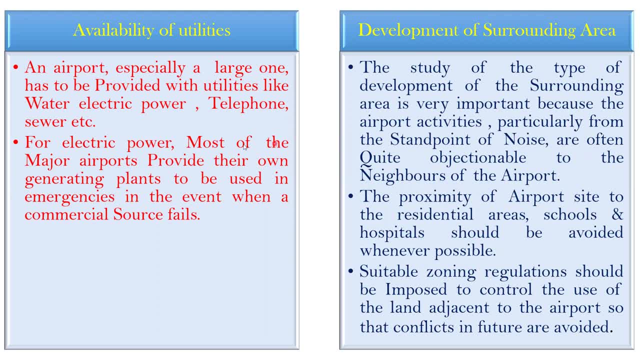 avoided, right? We've already seen this as well. right, Because if you're putting up an airport, so next to that we are to do proper sound and air connection. So, for example, if you are having a, we have to do proper zoning so that what will happen? the adjacent land, what we have? no, the 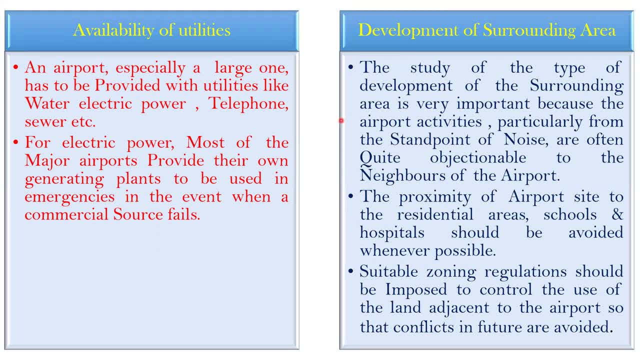 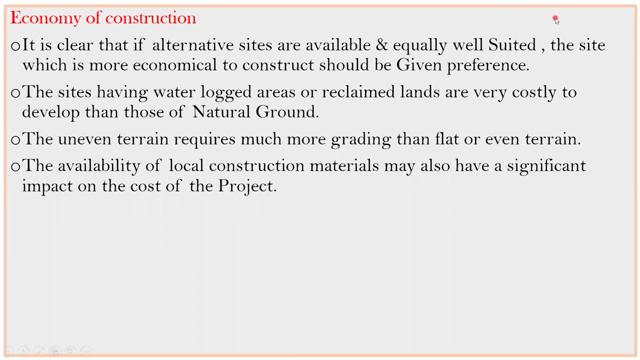 the proper zoning will be done and proper regulations will be uh, put up so that there is no construction happening and all right, so that in future those conflicts can be avoided. yeah, so next is economy of construction. it is clear that if alternative sites are available and equally well suited, the site which is more economical to construct should be given. 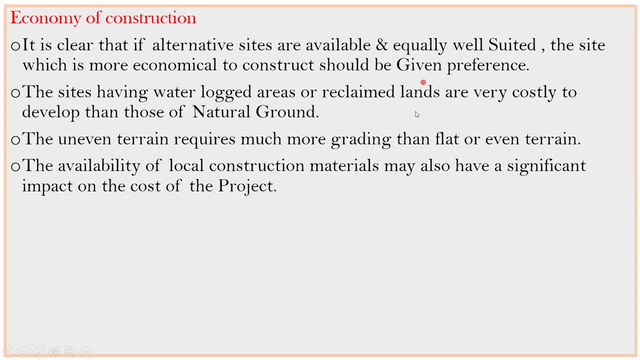 preferences. the sites having waterlogged areas or reclaimed lands are very costly to develop than those of natural ground. right suppose, if you have waterlogged areas and all, then the dewatering becomes a problem. then every now and then you have to do the dewatering and all which. 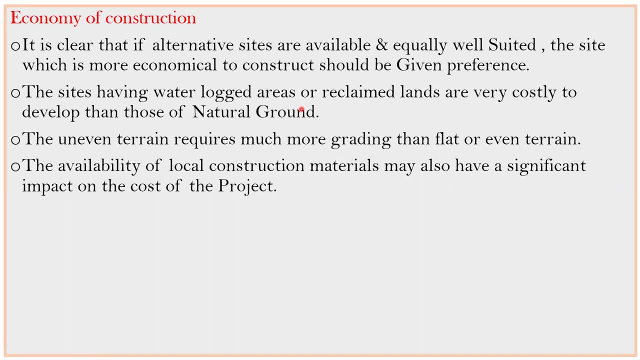 again, uh brings in the extra cost to the project. so as far as possible all these things should be taken into consideration. the uneven terrain requires much more grading than the flat or even terrain. right. let's say you have a land where the land is something, the terrain is something. 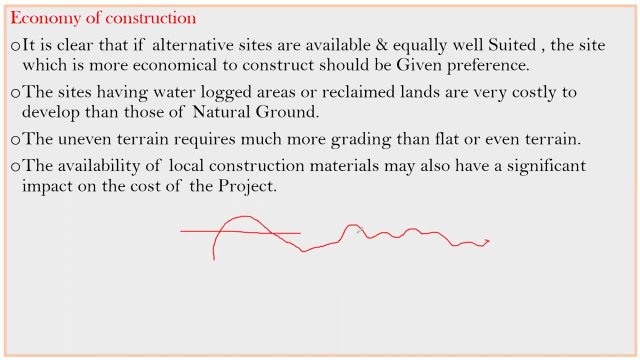 unbelievable. you don't know how much land you have to get to get to the right land to get to the right land. you don't know how much land you have to get to the right land to get to the right land. you don't know. and down in this way, then what will happen? if you want to put a flat terrain, then what will happen? 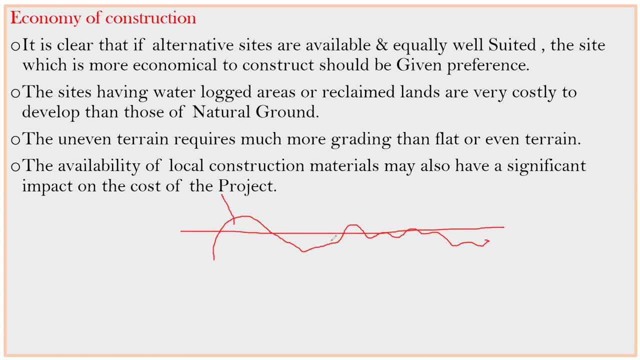 this much portion. you have to do the cutting here. they have to do the filling right. so in this way what will happen? you have to do more and more grading. so again it's the additional cost. so that is where the uneven terrain requires much more grading than flat or even terrain. the last 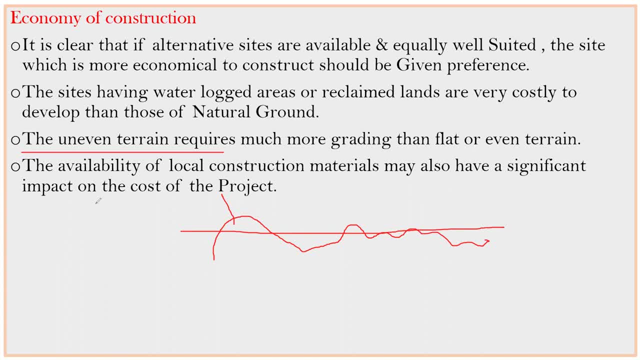 is, the availability of the local construction materials may also have a significant impact on the cost of the project. right, whatever materials we require for this project to carry out, they should be locally available in the surrounding uh radius of, let us say, one or two kilometer if. 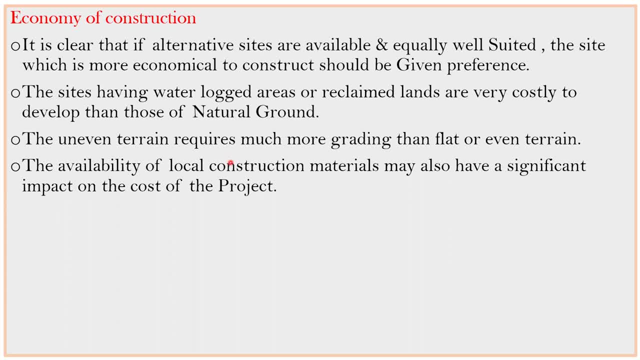 it is not available, then if you want to bring it from the place, let us say 10, 15 kilometers from there, again that will- uh, you know, will- again that will lead to the extra cost for the project. so all these things we need to consider, yeah. the next is presence of other airports. the airport should be. 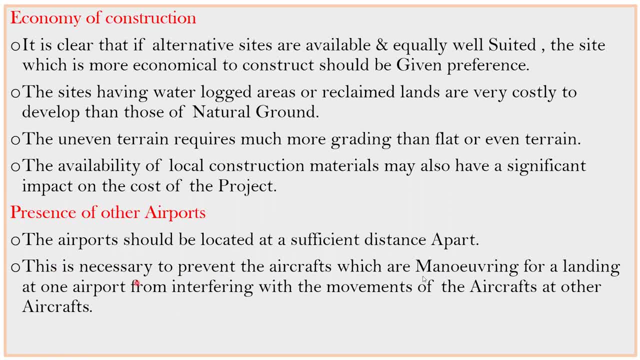 located at a sufficient distance apart. this is necessary to prevent the aircraft which are maneuvering over a landing at one airport from interfering with the movements of the aircraft at other aircrafts. so this also we know. as far as possible we should make sure there is a proper gap between the two airports. i mean you shouldn't try to construct. 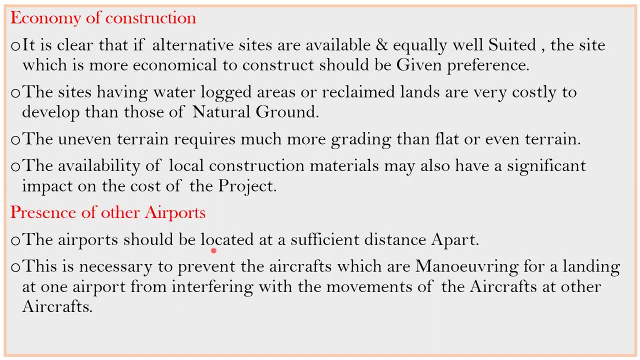 airports very close to each other right, so that will again effect in the takeoff and the landing of the airport. so as far as possible try to keep a sufficient distance apart. now, how much distance we need to keep apart, that is given here. so serving small general aviation aircrafts under. 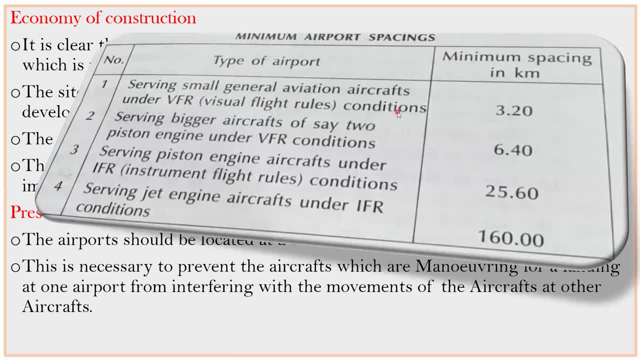 vfp. vfr stands for visual flight, flight rules conditions serving bigger aircraft of, say, two piston engine under vfr conditions, then serving piston engine aircraft under ifr conditions and serving jet engine aircraft under ifr conditions. so these are different types of airport. what we have based on that it is given here minimum it has to be 3.2 kilometer. then if you are putting up a 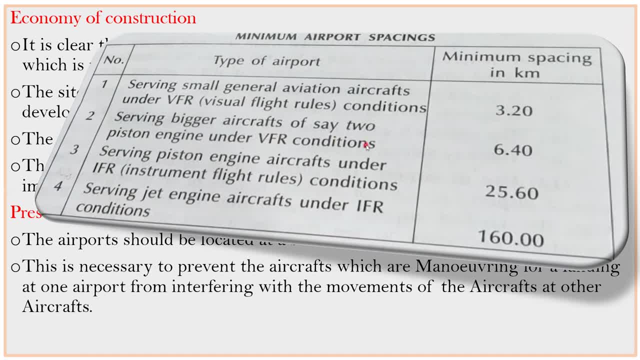 bigger aircraft of, say, two piston engine under the vfr condition, that is, visual flight rules, then it has to be 6.40 kilometer, then it is 25.60, and for serving the jet engine aircraft it has to be 160 kilometers. so all these are given by ico, that is, international civil aviation organization, and based on that all, 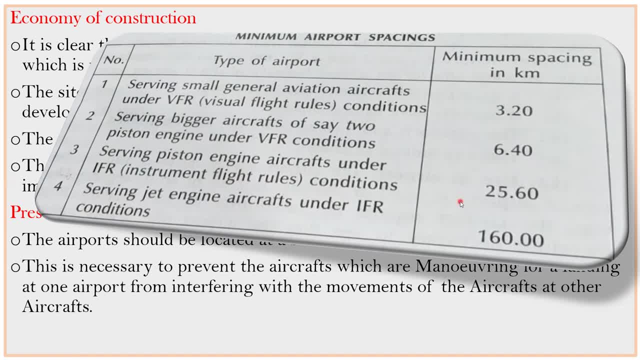 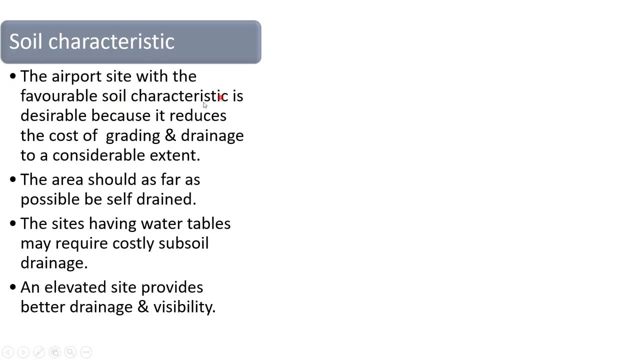 these things will be strictly followed whenever we construct any new airport. yeah, and the last is the soil characteristics. the airport site with the favorable soil characteristic is desirable because it reduces the cost of grading and drainage to a considerable extent. the area should, as far as possible, be self-drained. 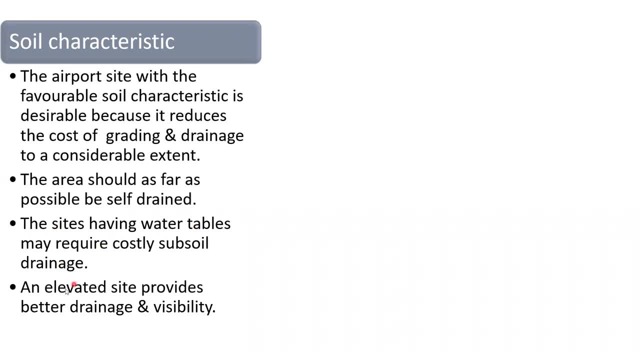 and the sites having water tables may require costly subsoil drainage, and elevated site provides better drainage and visibility. we have seen that if the soil is good, then the proper drainage and all is going to happen so that it would be easy for us for the construction. and the last is a 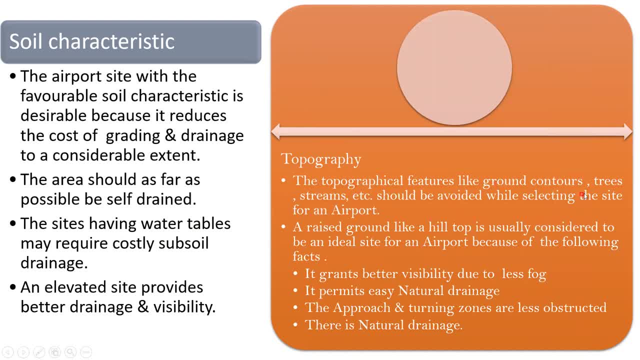 topography. the topographical features like ground contours, trees, streams, etc. should be avoided by selecting the site for an airport. a raised ground like a hilltop is usually considered to be ideal site for airport because of the following factors. the first is that if you're putting a, i mean if you're using a raised ground hill top, then it 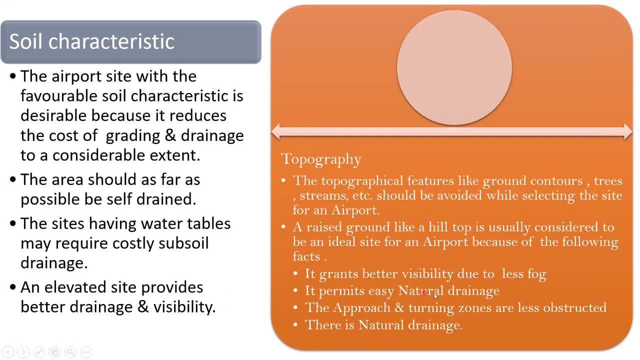 grants a better visibility due to the less fog. it permits easy natural drainage. since it's at the top, the water is not going to stay there, it's going to flow from there right. so it permits permits easy natural drainage. the approach and turning zones are less obstructed and there is a natural drainage. 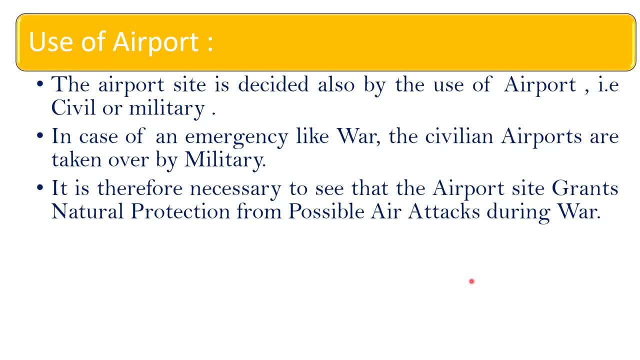 and the last is the use of airport. so what exactly? what airport exactly you want to put up the airport? so the airport site is decided also by the use of airport, that is, civil or military. in case of emergency, like war, the civil airports are taken over by the military, and it is therefore necessary. 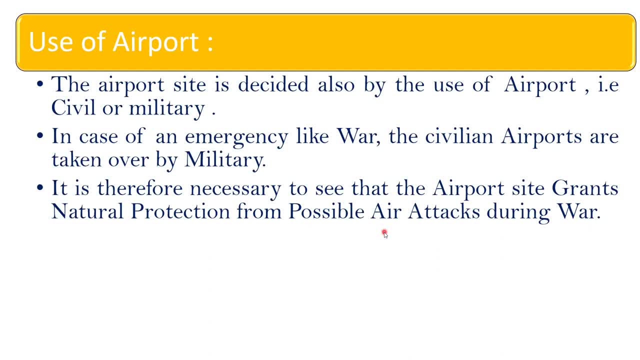 to see that airport site grants natural protection from the possible air attacks during the war right. so whenever we put the civilian airport also we'll try to keep that airport in such a location. so tomorrow, if you're using it for military, so that should have a natural protection from the air. 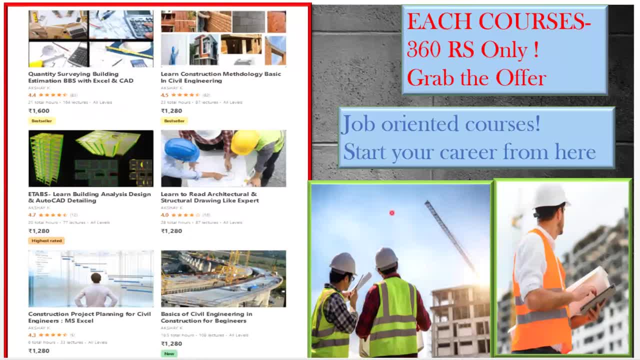 attacks during the war and on. yeah, so this was all about the airport and we will be seeing you again in the next video. Bye, bye. criteria that we need to consider for the selection of the airport, or almost 8 to 10 criterias that we need to consider, and there are a lot of points that we have understood.